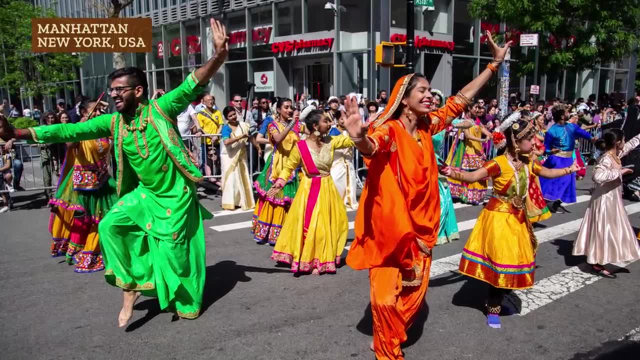 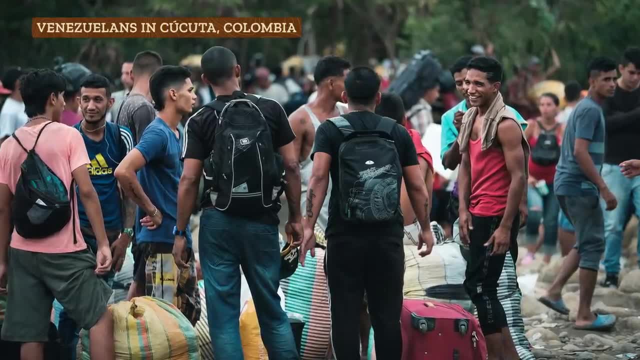 of India And today we see elements of Indian culture all over the world. Moving that many people and creating those cultural melds didn't just happen overnight. People have been migrating and transplanting since before recorded history And understanding the reasons people migrate can. 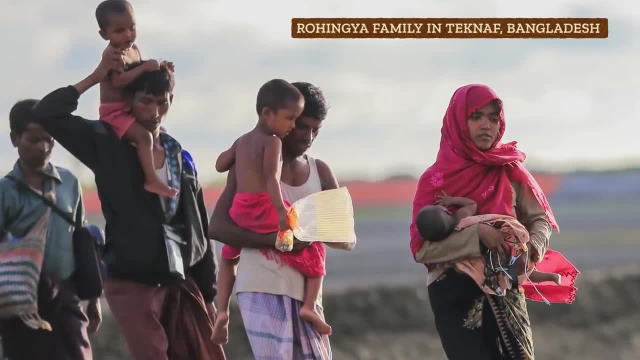 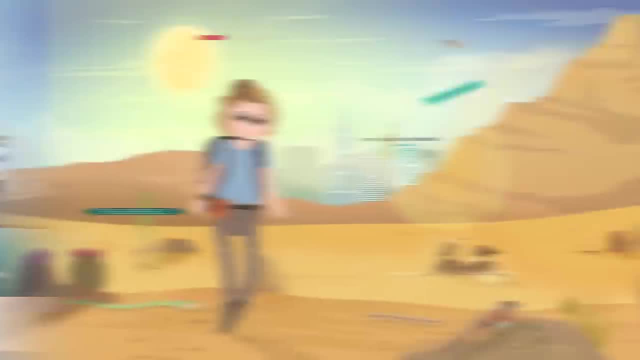 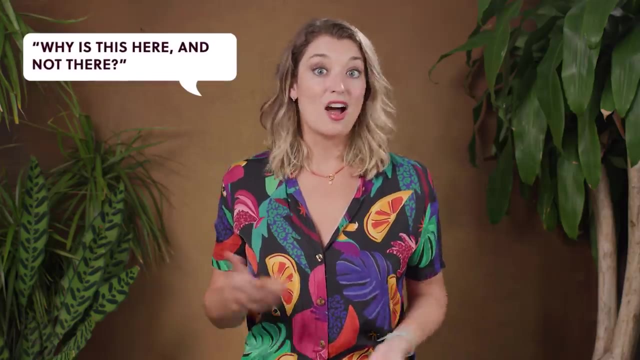 help explain some of that. So let's get started. the cultural and even economic and political patterns we see around the world. I'm Alizé Carrère and this is Crash Course: Geography. After asking, why is this here and not there? in geography, our next big question is: 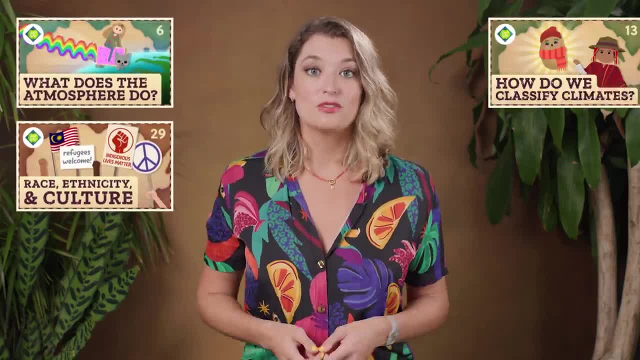 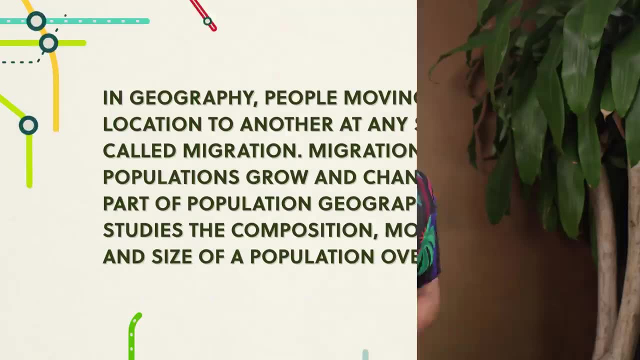 how did this get here? From air pressure to Malaysian architecture, to potatoes and bananas, geographers study the movement of just about anything on the planet Or off, but that's another series In geography. people moving from one location to another at any scale is called. 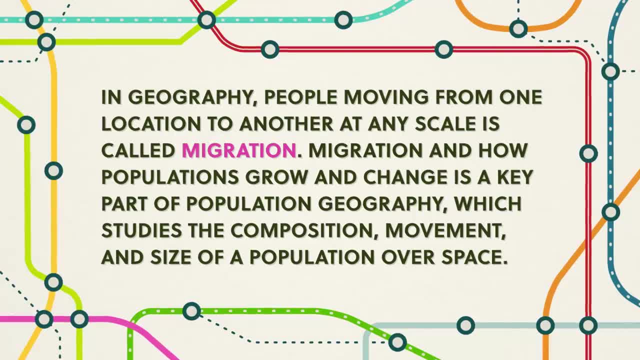 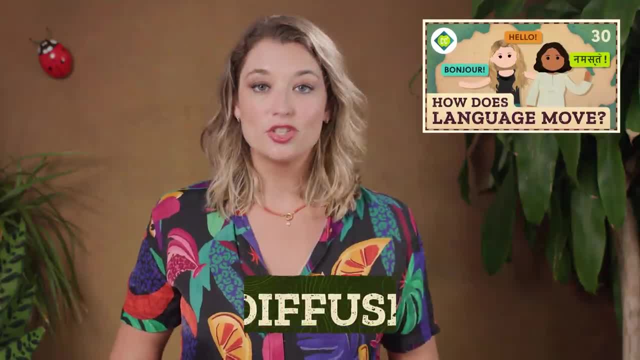 migration. Migration and how populations grow and change is a key part of population geography, which studies the composition, movement and size of a population over space. Much like ideas and innovations diffuse, people move too. So for the next 2 episodes we're going. 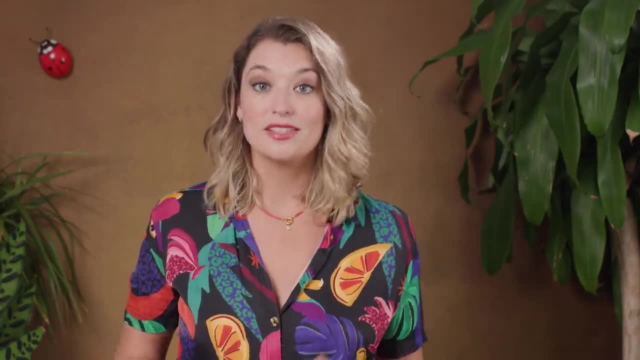 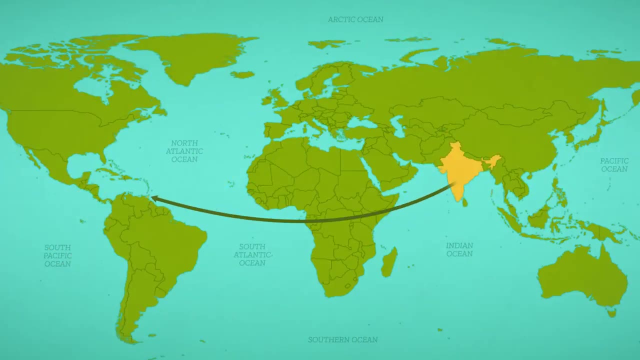 to examine how populations move and change and some of the consequences of those movements. Let's start by exploring how people from India made it all the way to the Caribbean islands of Trinidad and Tobago. It's a challenge for most of us to understand where they are. 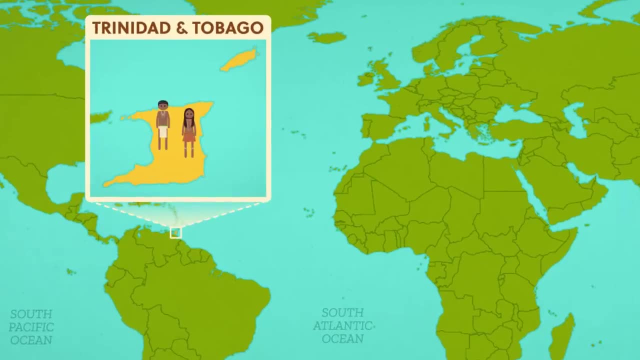 complex story. Originally, the islands were home to the Arawak and Carib-speaking peoples, But through war, slavery and intermarriage this population had largely been eradicated or assimilated by the time sugar plantations were started on Trinidad by the Spanish in the 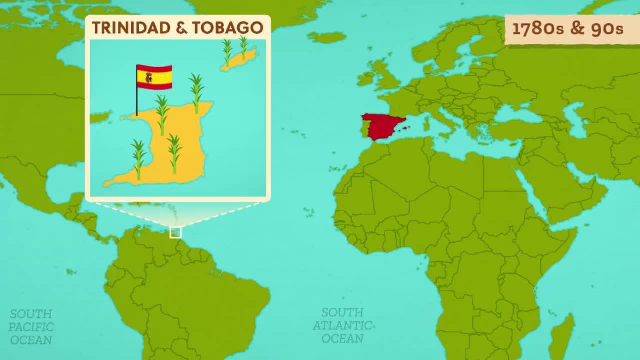 1780s and 90s. So, in order to operate the plantations, people from West Africa were enslaved and underwent forced migration to the islands. Then, in 1834, the British, who now controlled the island of Trinidad, outlawed slavery throughout the British Empire. 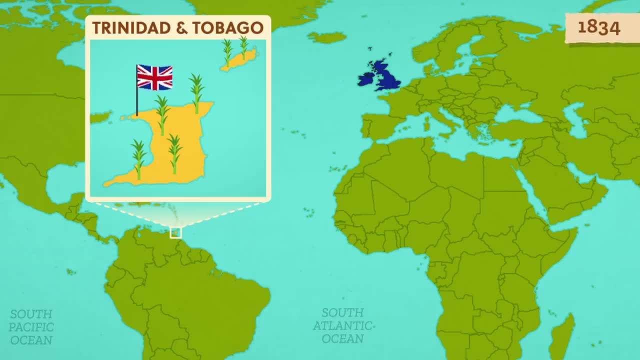 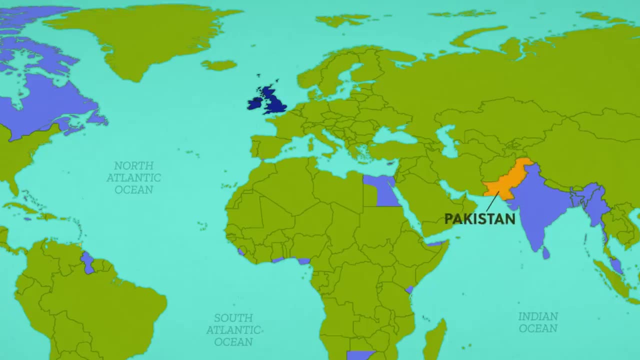 So the British government needed to find a new way to bring cheap labor to the plantation fields. At this time the British colonial empire was vast and included control over most of South Asia, including the countries we now call Pakistan and India. So the British began advertising. 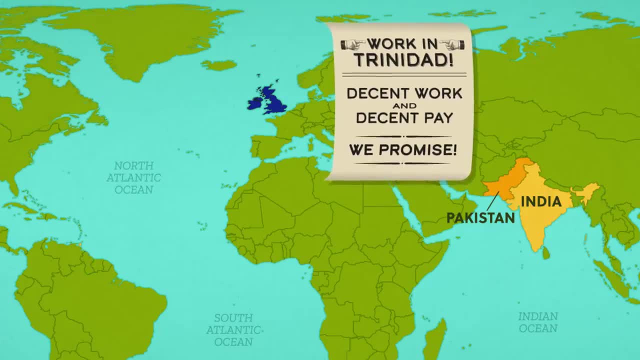 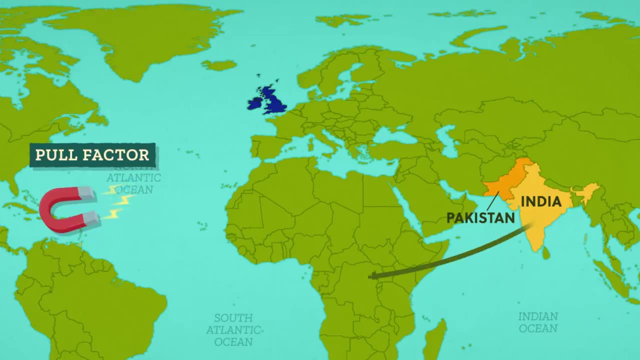 to Indians that they could come and work in Trinidad, promising them decent working conditions and pay. The promise of better wages was what in geography we call a pull factor. That means people moved because something pulled or attracted them to a new place, like better wages or a safer living environment. 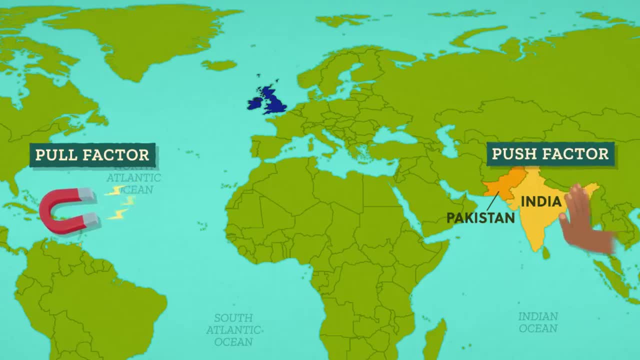 But people can also be motivated by a push factor, like the poor living conditions for some in India that pushed people to consider moving to Trinidad. This situation illustrates a type of economic migration, If a person lives somewhere where it's difficult to make a living. 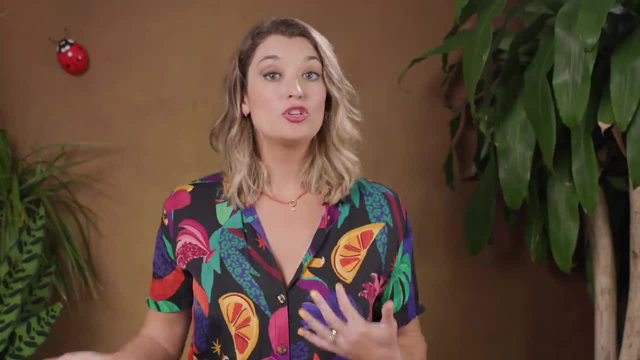 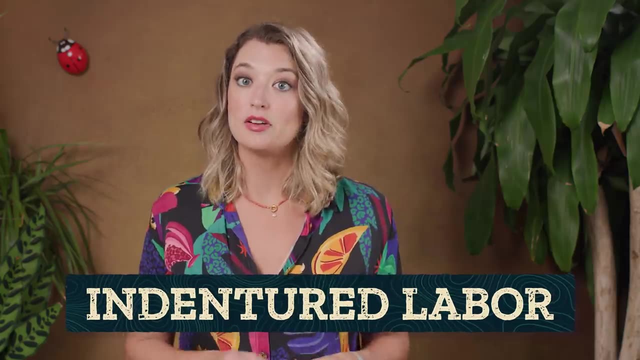 they're more likely to look elsewhere to find new opportunities. So, pushed and pulled from India, people migrated to Trinidad as indentured labor, where they were contracted to work for low pay on an estate for a set period of time, often for years, and often as a way to pay off the cost of their travel to the new place. 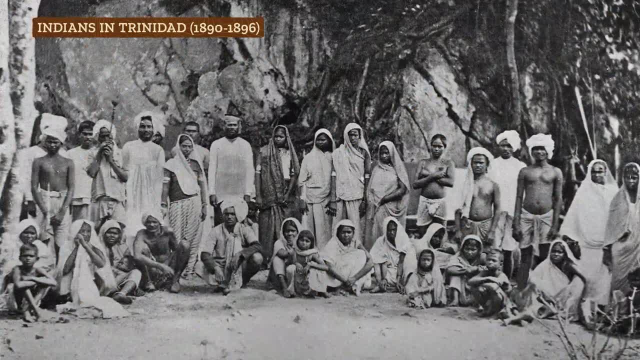 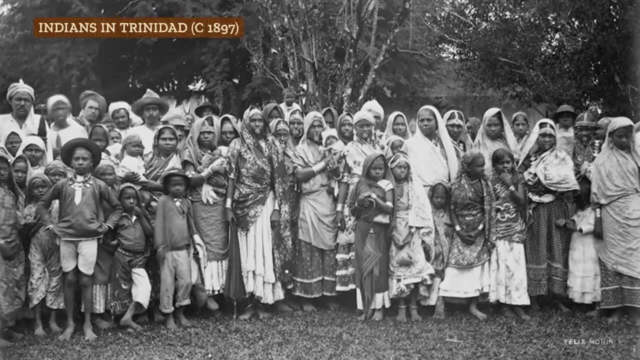 Indentured labor can be considered a sneaky way to enslave someone without calling it slavery, but there seems to be some evidence that, at least in Trinidad and Tobago, there were a wide range of outcomes. Some Indians were able to go back to India with saved income. some Indians bought land to stay on the islands. 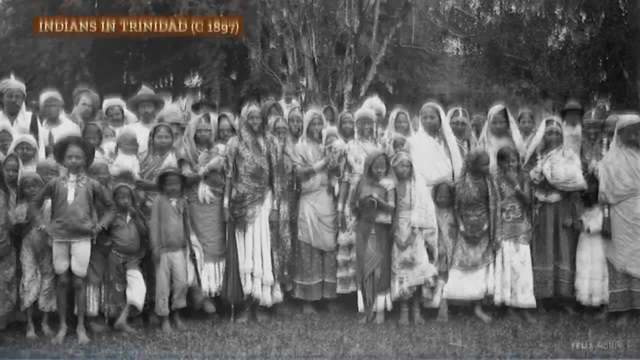 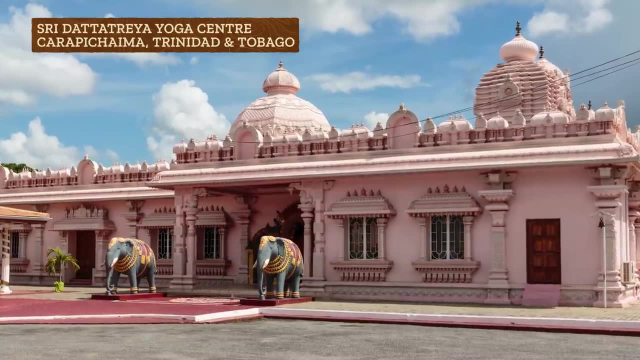 and some were treated horribly, wanted to go home and weren't able to Because so many Indians remained on the islands and mixed their cultural traits and families with the people of West African and British descent who also migrated there. it created a unique Creole culture. So we'll see Indian food with West African and other twists. 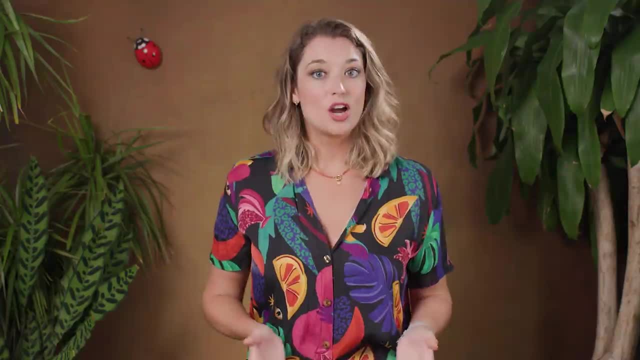 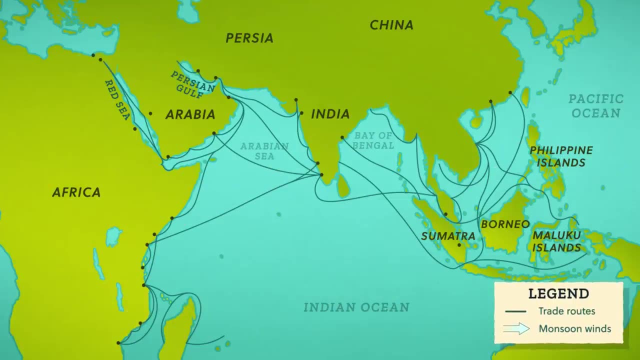 and music that blends elsewhere with the culture. But what this means is that most of elements of all of these cultures. But the 1800s were far from the first time Indians left the subcontinent and migrated. We have records going back at least 2,000 years and some say 3,000 years. that monsoon. 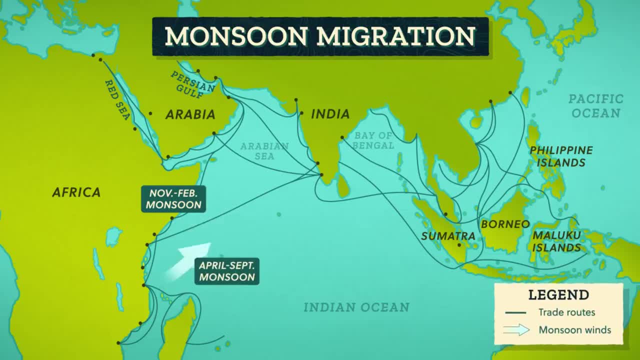 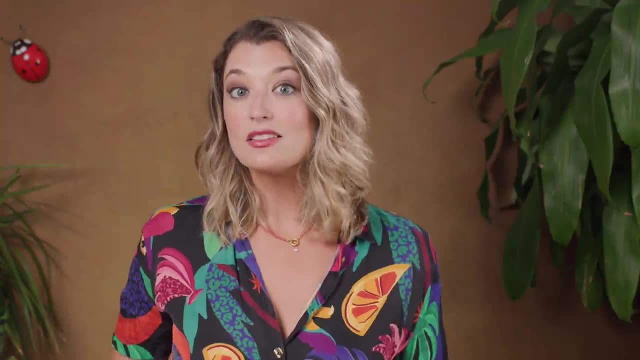 migration driven by the monsoon winds was happening between India, the Persian Gulf and East Africa. This seasonal or cyclical migration happens when people migrate in a back and forth pattern, And we see this a lot in migration tied to agriculture, where work depends on harvest. 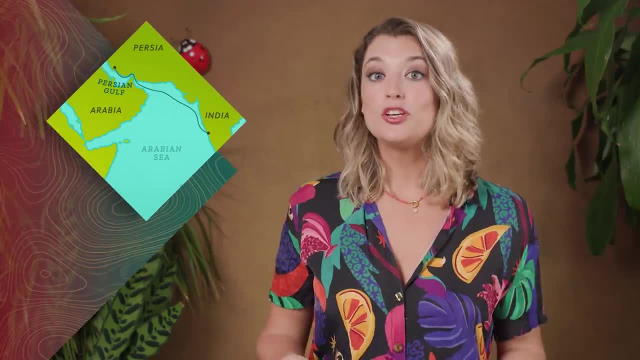 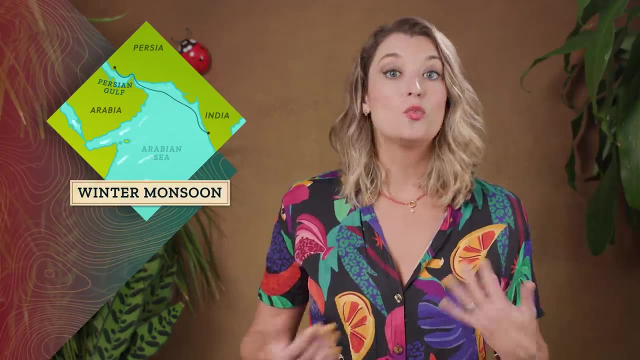 seasons or, in this case, transportation patterns, Pulled to new regions by the promise of trade and profit, sailors would leave the west coast of India and ride the prevailing winds to the Persian Gulf. Then, as the winds shifted months later, the sailors would sail back to India. 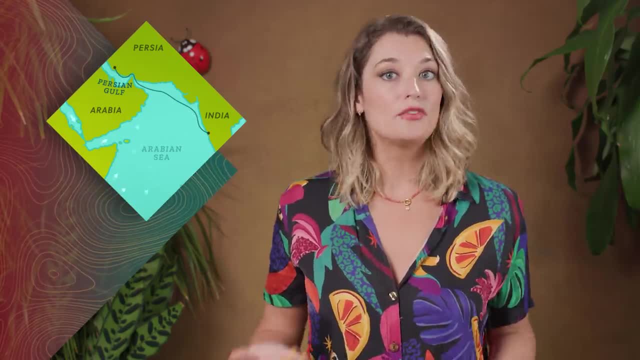 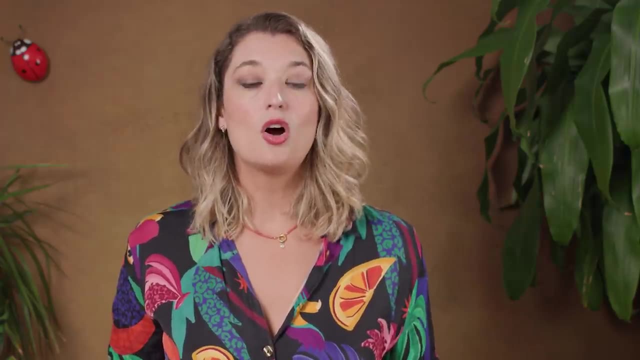 And because of how long the sailors would stay between wind shifts. traditions were often shared, as well as innovations and goods, But while trade hubs and cultural enclaves grew in coastal places like Tanzania, East Africa also holds a history of forced or involuntary migration. 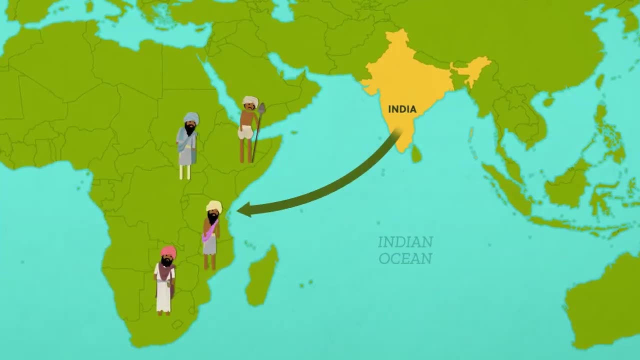 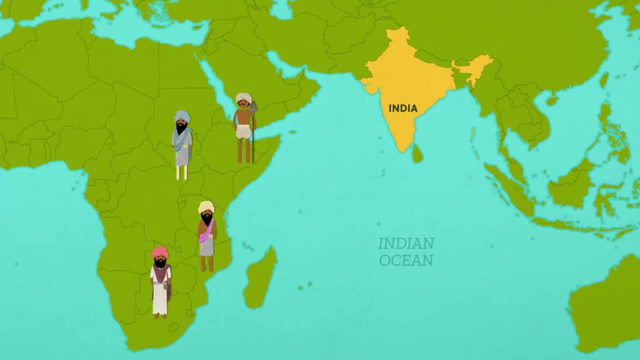 Either as enslaved people or indentured labor. the British would use Indians to create a class of people to own the land, Or as slaves to oversee the Africans in Africa and for manual labor. As slavery and servitude ended in the 1800s, many Indians stayed in the only home they 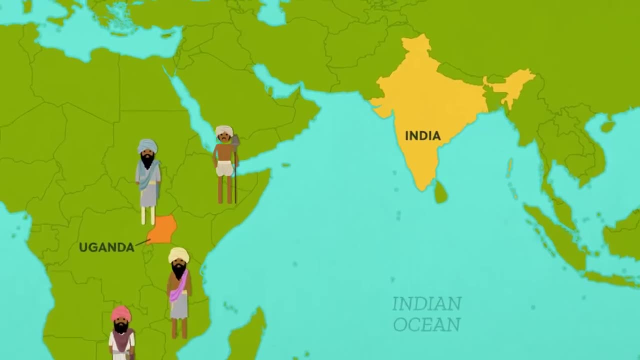 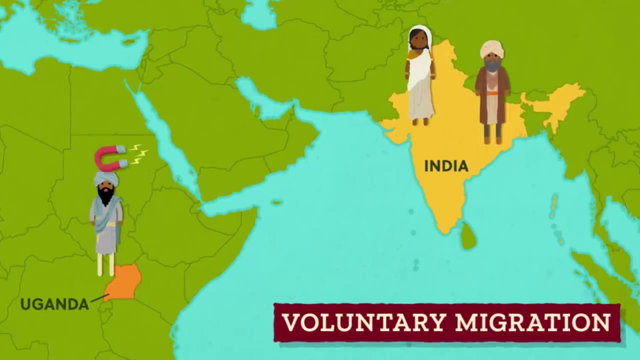 knew places like what's now called Uganda and South Africa. They then encouraged a wave of voluntary migration or the movement and settlement of people of their own choosing. People were pulled to stay in Uganda and pulled other people from India to come join them. 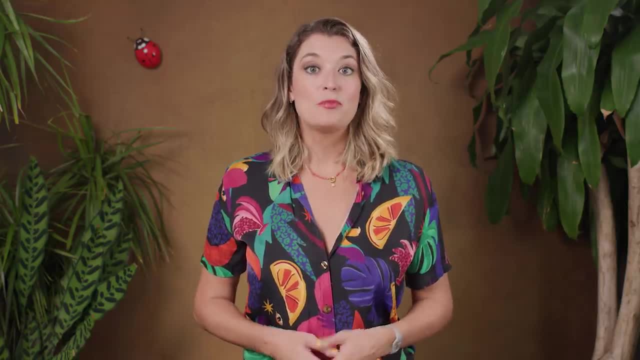 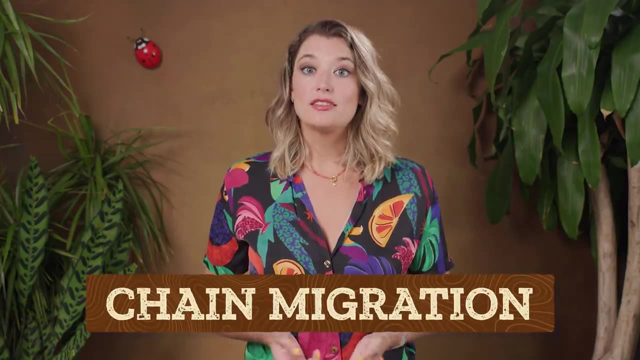 At first this movement to East Africa was mostly men, but over time, with people wanting to make the trip back to India less frequently, other people eventually joined the men to create families there. Chain migration like this reduces the uncertainty of migration because those moving to another 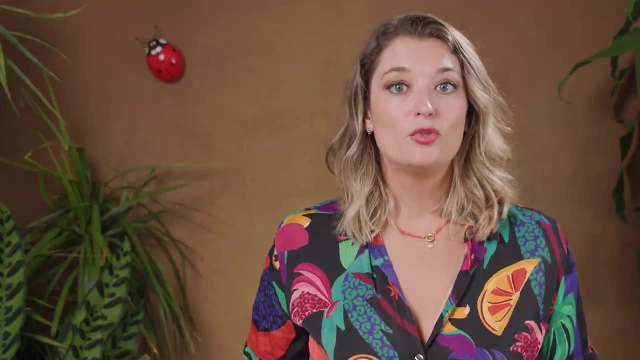 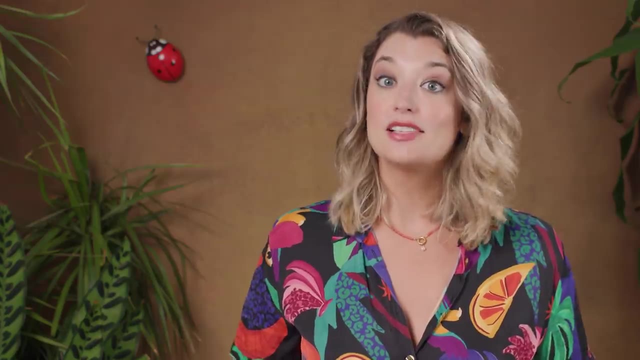 place join others in their existing network. In particular, Uganda was one place where people of Indian descent wove themselves into the community throughout the 1800s. They became business leaders and set up schools And place names in Uganda, like Shimoni Road, named for the Shimoni Islands, which are a 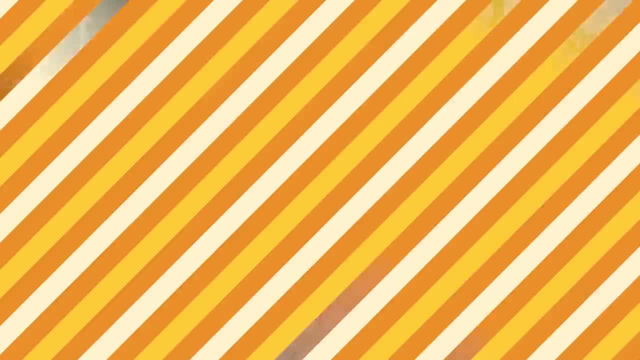 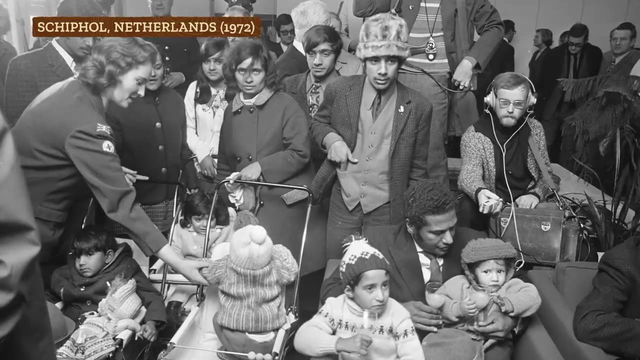 part of India even reflected elements of Indian culture. Indians were part of a Ugandan culture for at least 100 years, but that doesn't mean they were accepted in the country's culture. They were part of the country they lived in. In August of 1972, most Indians were expelled by the Ugandan military leader, Idi Amin, and 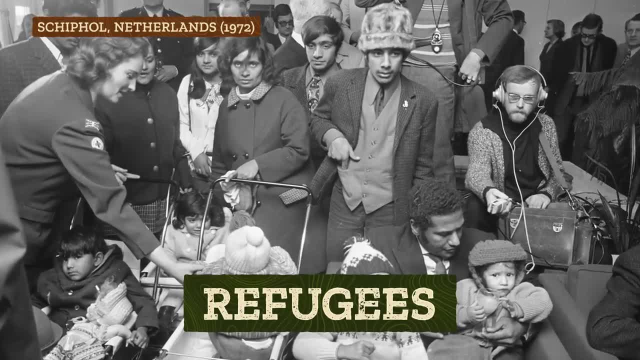 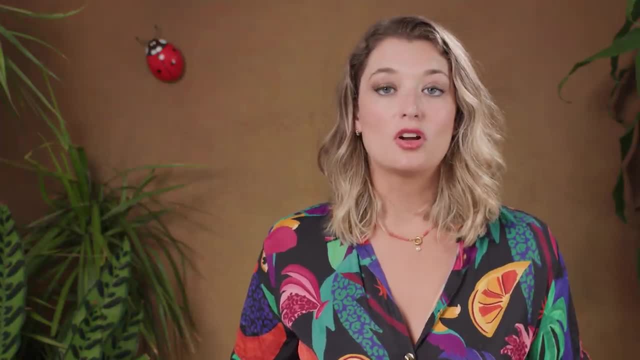 became refugees or someone who no longer feels safe in their home due to conflict or persecution and has to move. India didn't claim most of those forced to leave as Indian citizens. Many of them had lived in Uganda for a couple of generations and they didn't identify. 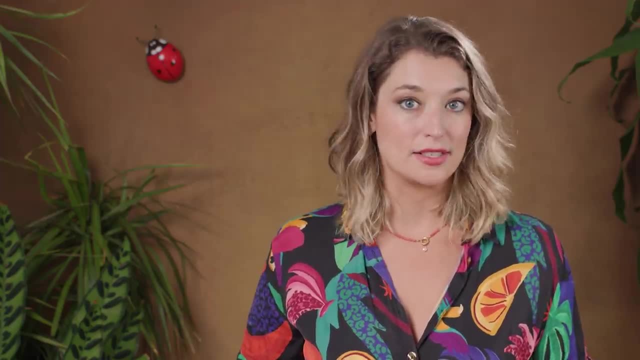 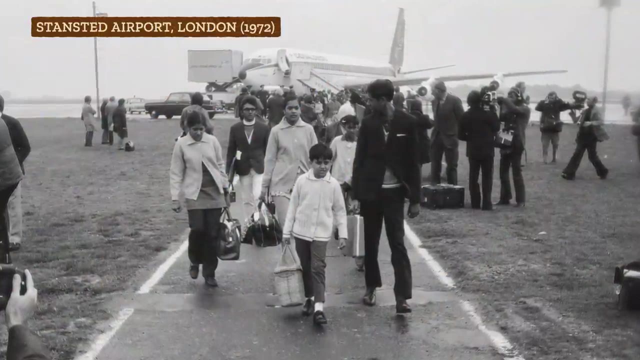 with the country that shared their physical features or even some of their cultural practices. Instead, over half of the 55,000 Indians being expelled had British passports and were able to relocate to the United Kingdom, And others were able to find homes in neighboring countries like Kenya, where some refugees 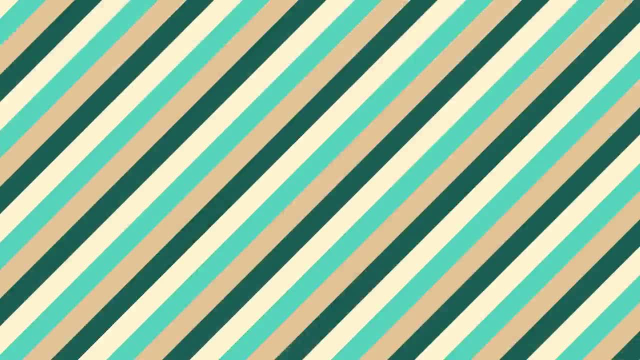 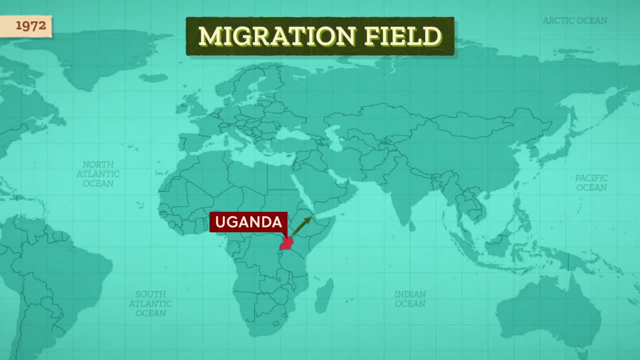 settled until it was safe for them to return to Uganda in 1986.. Where a nation of people moves to is called the migration field. In this case, the migration field of those expelled from Uganda in 1972 included India, Kenya, other countries with British ties like Tanzania, and Great Britain itself. Like many of these refugees, when someone is deported or removed from a country they call home, they often have nowhere to go. However, return migration can occur when a person goes back to stay in their country, to stay in their country of origin or citizenship. 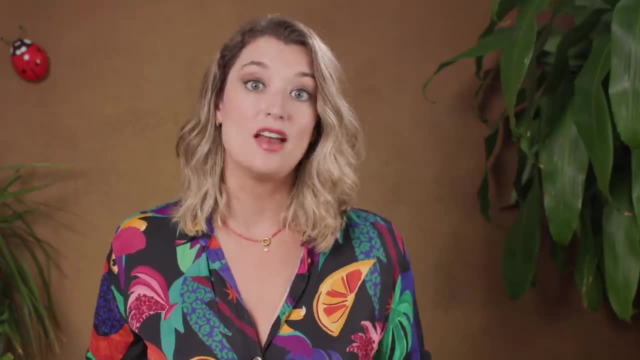 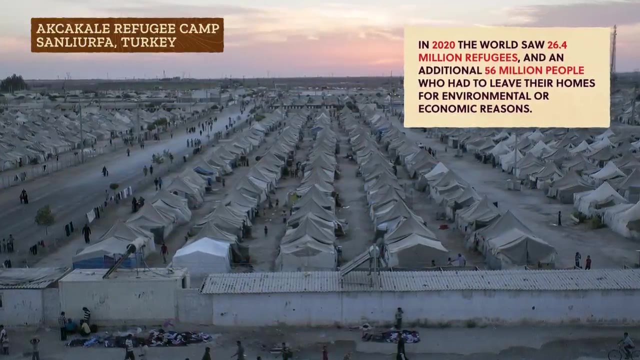 Like those with British passports, were returned to Britain, even though most of them had not lived there before. In 2020,, the world saw 26.4 million refugees and an additional 56 million people who had to leave their homes for environmental or economic reasons. 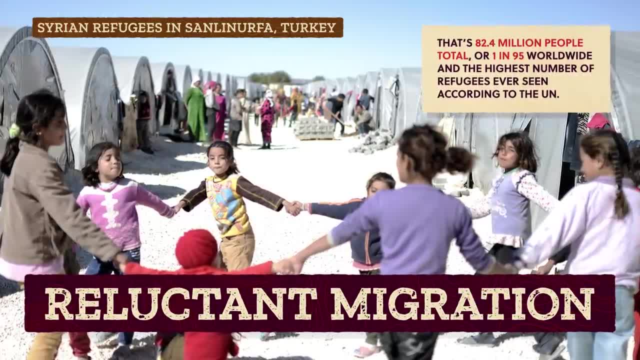 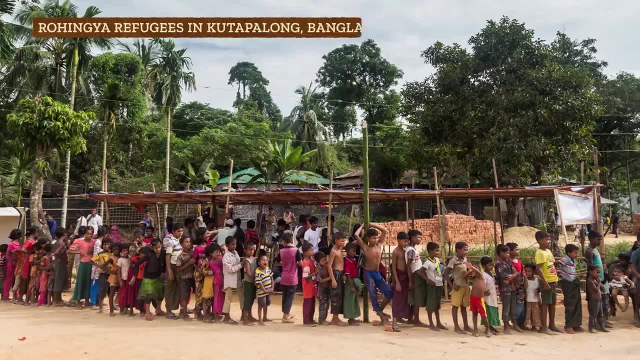 Refugees are a part of reluctant migration or people who feel they must move for safety reasons or are pushed by a fear of death if they stay Increasingly. climate change is one of these factors pushing people to migrate. Refugees are supposed to have protected status. 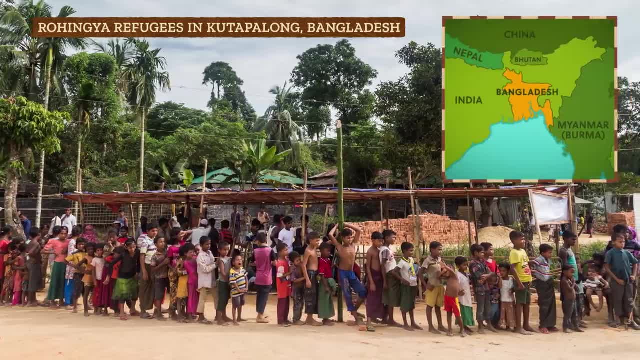 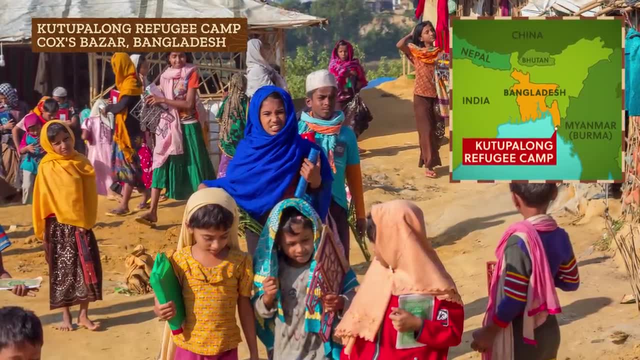 But as unlivable situations become increasingly widespread, there are a lot of refugees in the world right now. Refugee camps like Kudu Palang outside of Cox's Bazar in Bangladesh are supposed to be temporary but can become permanent. International organizations like the United Nations attempt to create international protections. 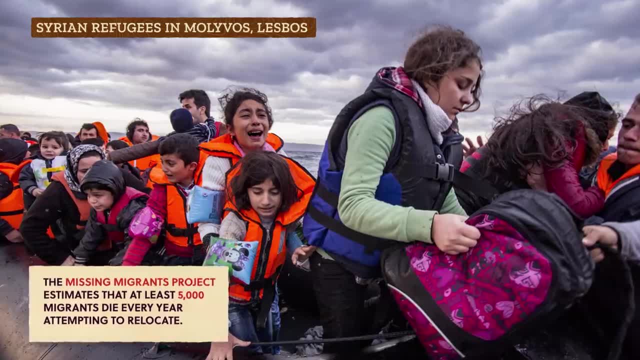 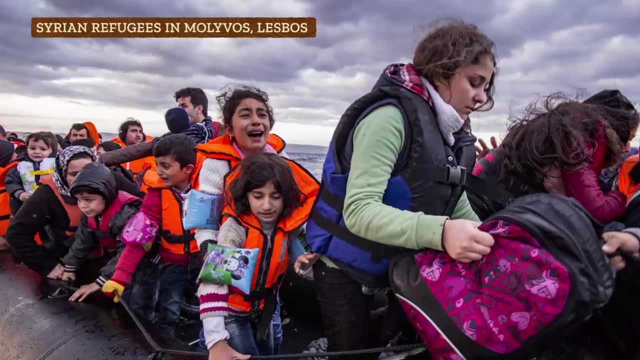 for refugees to provide safe migration routes. Despite those efforts, the Missing Migrants Project estimates that at least 5,000 migrants die every year attempting to relocate. For some people, the push factor of risk of immediate death at home is worth the risk. 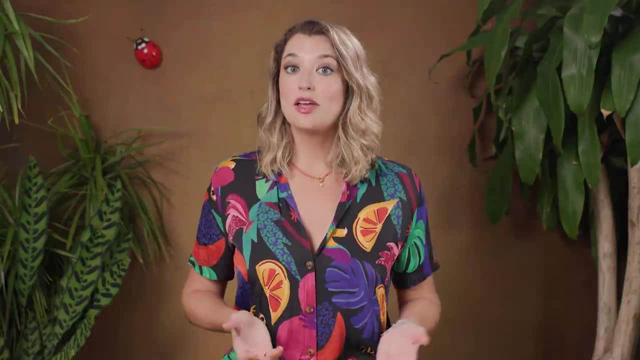 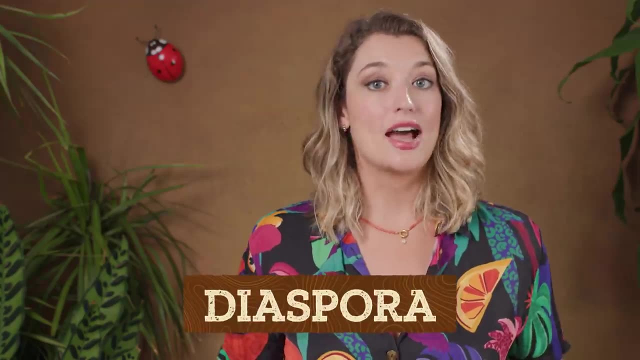 to try and reach a safe country in which to rebuild their lives. So just today we've seen there are millions of Indians living in the Caribbean, in the United Kingdom and in the Middle East and East and South Africa. This is called a diaspora. 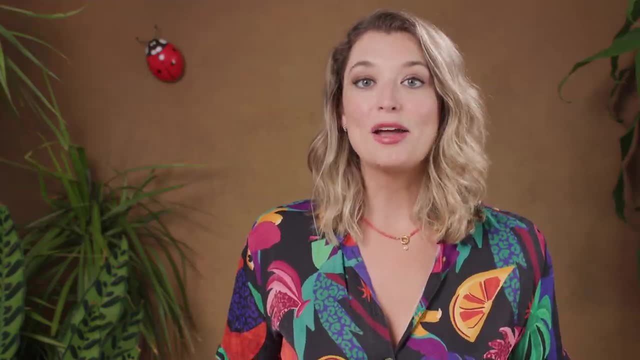 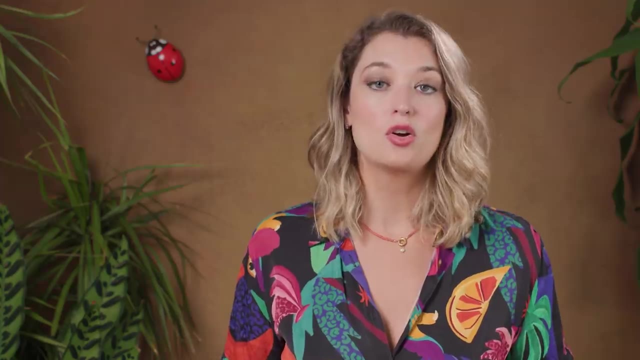 In fact, the Indian diaspora is the largest in the world And, while migration is the movement of a person from one place to setting up a home in another place, a diaspora indicates that a nation or people who share a cultural trait has. willingly or otherwise left their homeland. The people in a diaspora may not have been born in the place they have a cultural affinity for, But at a global level there's a desire to keep a cultural or even physical connection to that place. Some people even describe it as a longing to return home, even if there isn't a place. 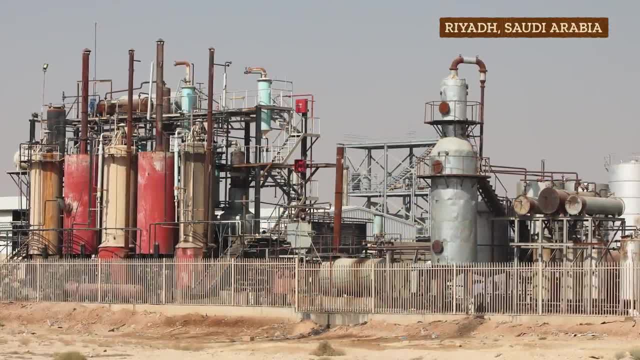 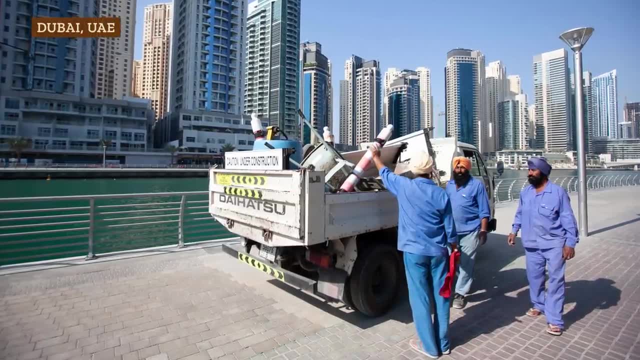 to return to In 2020, the bulk of Indian migrants are voluntary economic migrants working in a wide range of places, including the Persian Gulf. That millennia-long relationship continues today, with Indian workers mostly working in oil fields and other manual jobs like caregiving and cleaning. 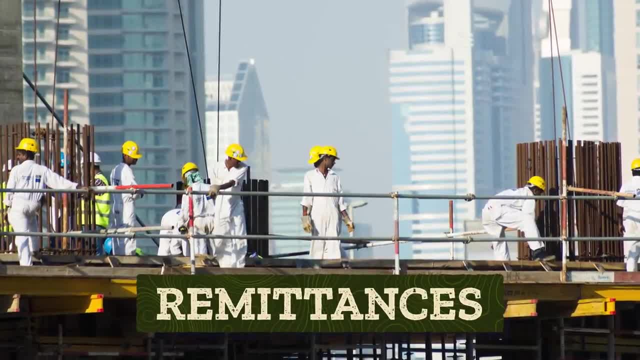 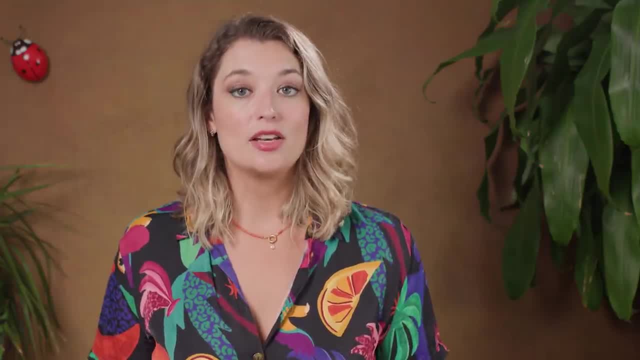 The workers are majority male and they send money home as remittances to help their family access greater economic opportunities. But as oil and gas prices continue to rise, there's also a desire to keep a cultural connection. As oil prices fall and oil demand decreases, fewer Indians are migrating to the Gulf, which will change the international migration field and economies based on remittances yet again. While all of these types of migration sound large and dramatic and receive the most political attention, most migration actually occurs within the same country: Internal migration, like this has often happened as people from rural spaces are pulled to. 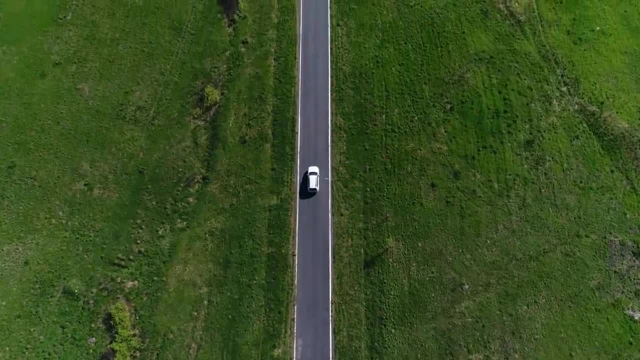 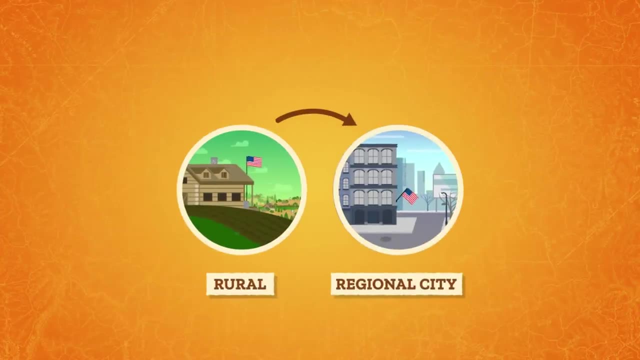 the economic opportunities in urban spaces where there may be more available jobs. In cases that aren't a matter of war or disaster, migration patterns often start from rural spaces. Migrations often start first with a move from rural to urban, then maybe from a regional. 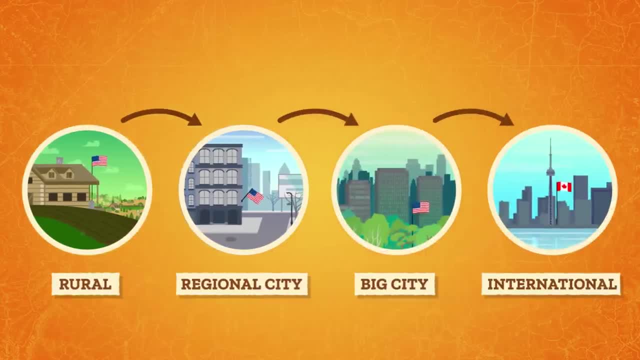 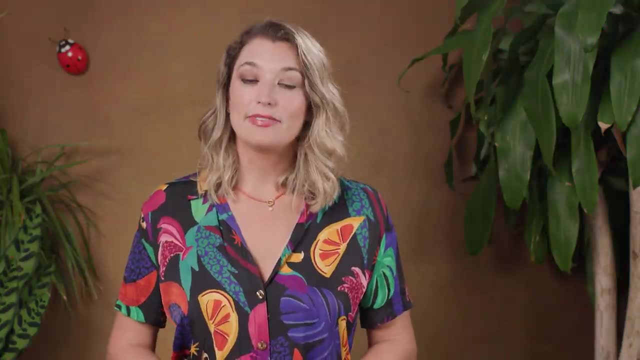 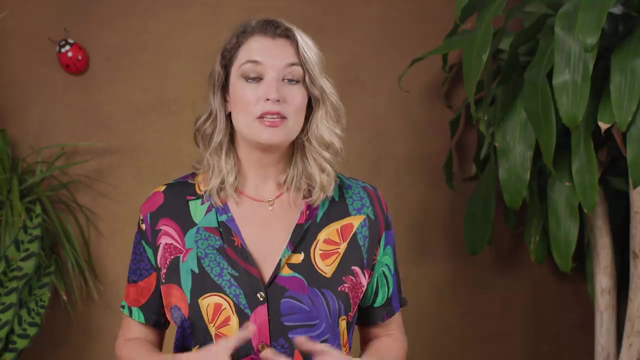 urban center to a bigger city within the same country and then a move internationally. This is called step migration, when a person makes moves that are more and more drastic. But even step migration, like all migration, is fairly risky. Many migrants only migrate internationally when they feel they have no other option.